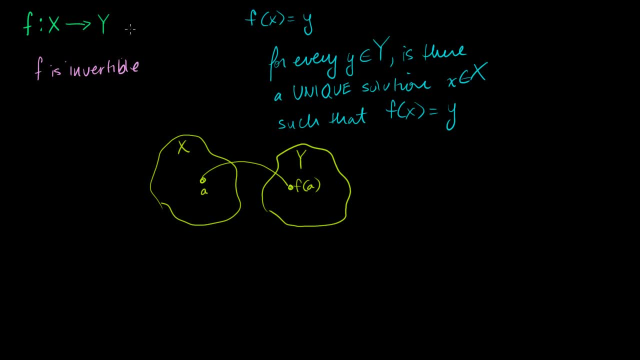 This is so far what just this tells us. Now I want to look at this equation here and I want to know that if I can pick any y in this set or any lowercase y in this set, y- so let's say I pick something here. let's say: 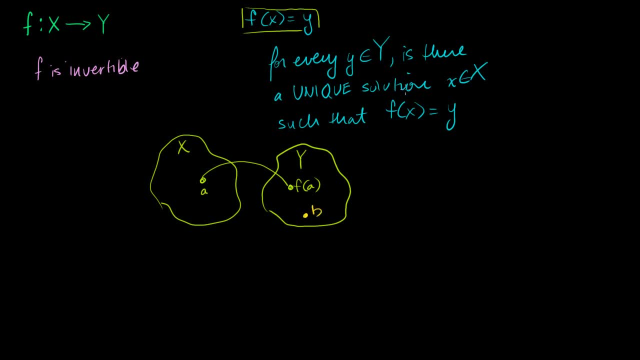 that's b. I want to know: is there a unique solution to the equation f of x is equal to b. Is there a unique solution? So one I guess you have to think: is there a solution? So is there a solution to this saying? look, is there some x. 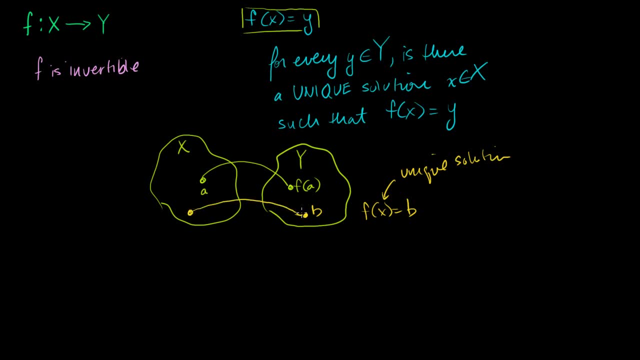 here that if I apply the transformation F to it, that I get there. and I also want to know: is it unique? For example, if this is the only one, then it's unique, but it's not unique if there's some other guy, if 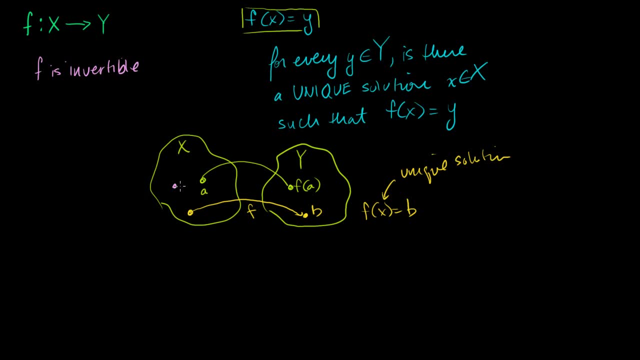 there's more than one solution. There's some other guy in x that if I apply the transformation, I also go to b. This would make it non-unique. Not unique, Yeah, not unique. So what I want to concern ourselves with in this video, 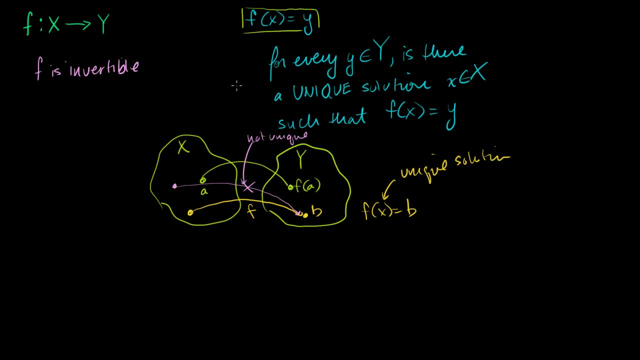 is. somehow is invertibility related to the idea of a unique solution to this for any y in our codomain. So let's just work through our definitions of invertibility and see if we can get anywhere constructive. So, by definition, f is invertible. implies that there 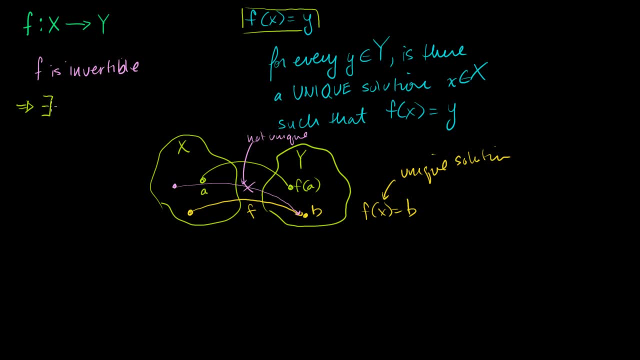 exists, this little backward-looking 3-looking thing. this means there exists. I think it's nice to be exposed sometimes to the mathy notation, so let me just write: there exists, That means that there exists some function. Let's call it f inverse. that's a mapping from y to x, such: 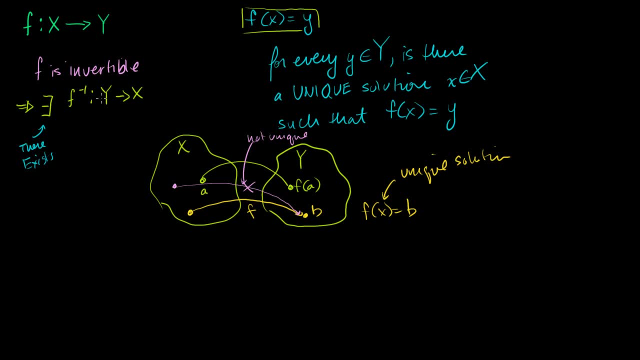 that, and actually the colons are also the shorthand for such that. but I'll write it out such that the composition of f inverse with f is equal to the identity on x. So essentially it's saying: look, if I apply f to 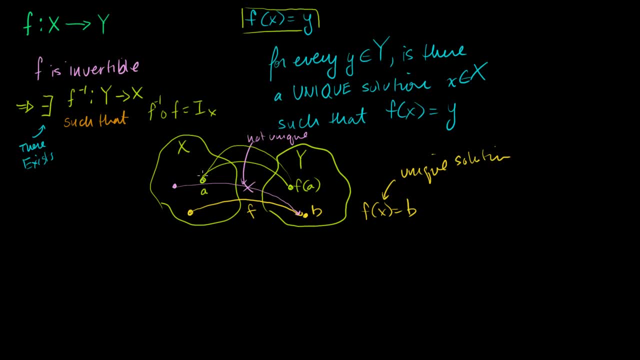 something in x, and then I apply f inverse to that. I'm going to get back to that point, which is essentially equivalent, or it isn't just essentially equivalent, it is equivalent to just applying the identity function. So that's ix. 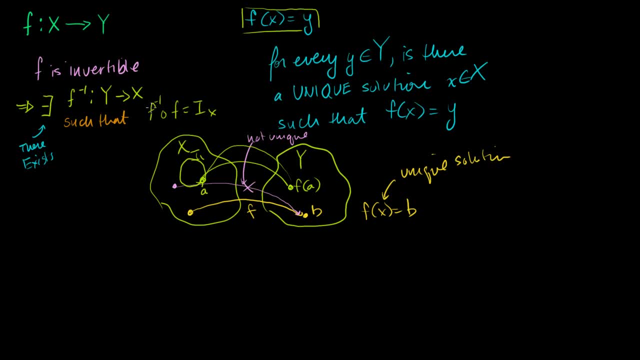 So you just get what you put into it, Such that this inverse function, the composition of the inverse with the function, is equal to the identity function, And That the composition of the function with the inverse function is equal to the identity function. on y. 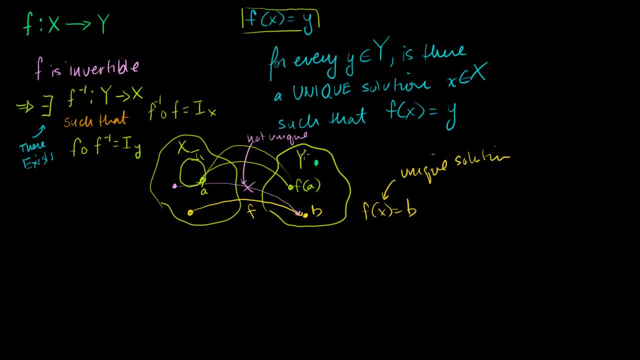 So if you start in y and you apply the inverse and then you apply the function to that, you're going to end up back in y at that same point, and that's equivalent to just applying the identity function. So this is what invertibility tells me. 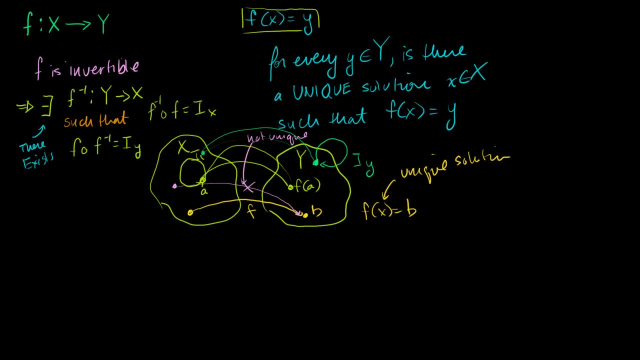 This is how I defined invertibility in the last video. Now we're concerned with this equation up here. We're concerned with the equation. I'll write it in pink: f of x is equal to y And we want to know for any y or any lower case cursive. 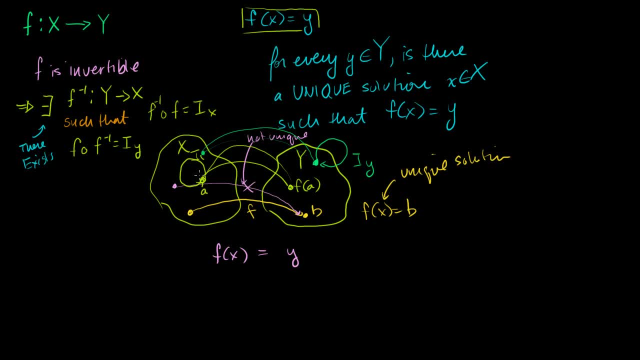 y in our big set y. is there a unique x solution to this? So what we can do is: we know that f is invertible. I told you that from the get go. So, given that f is invertible, we know that there is this f. 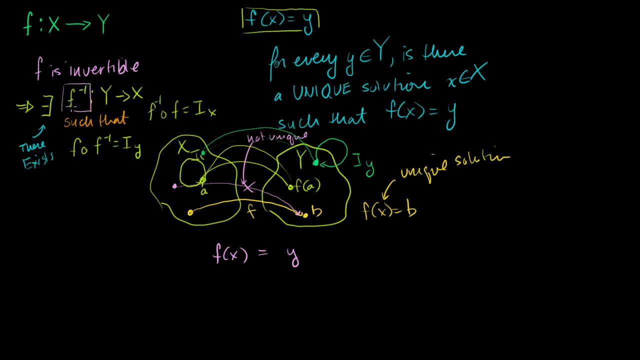 inverse function. We know that there's this f inverse function And I can apply that f inverse function. It's a mapping from y to x, So I can apply it to any element in y. So for any y, let's say that this is my y, right there? 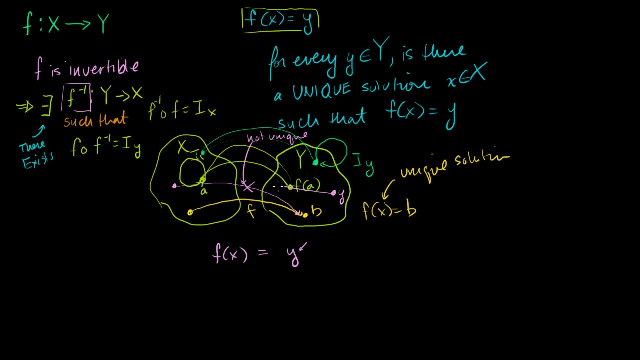 So I can apply my f inverse to that y- And I'm going to go over here- And of course y is equal to f of x. These are the exact same points. So let's apply our f inverse function to this. So if I apply the f inverse function to both sides of this, 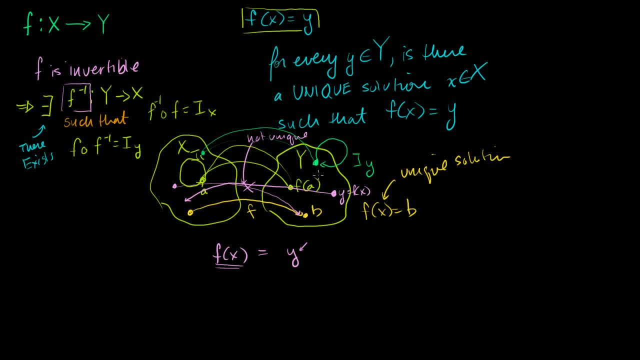 equation: this right here is an element in y And this is the same element in y. right, They're the same element. Now, if I apply the inverse mapping to both of that, that's going to take me to some element in x. 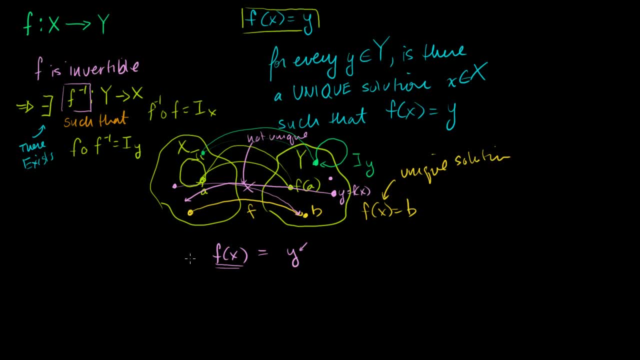 So let's do that. So if I take the inverse function on this, on both sides of this equation, Both sides of this equation- we have some element in x, We've got 2 f numbers over here in y and I'm taking the inverse function to get to. 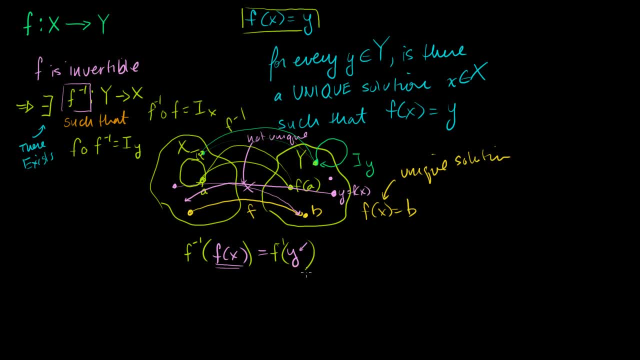 some element in x, And what is this going to be equal to? Well, on the right-hand side we could just write the f inverse of y. That's going to be some element over here. But what does the left-hand side of this? 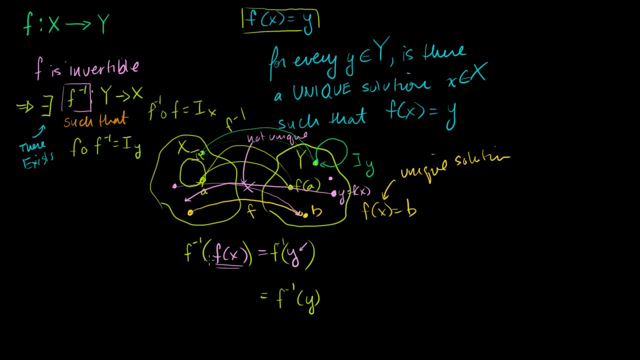 equation translate to The definition of this inverse function is that when you take the composition with f, you're going to end up with the identity function. This is going to be equivalent to. let me write it this way: this is equal to the composition of f inverse with. 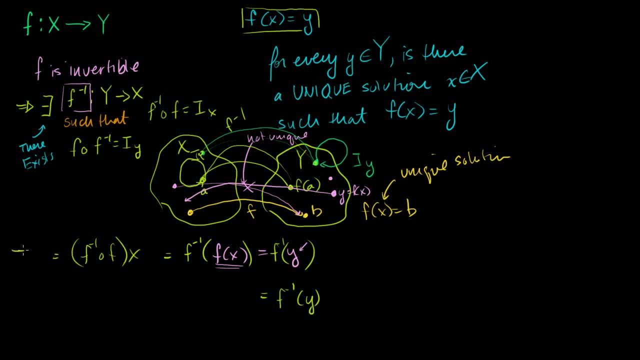 f of x, which is equivalent to the identity function being applied to x, And then the identity function being applied to x is what? That's? just x. This thing right here just reduces to x. This reduces to x. So we started with the idea that f is invertible. 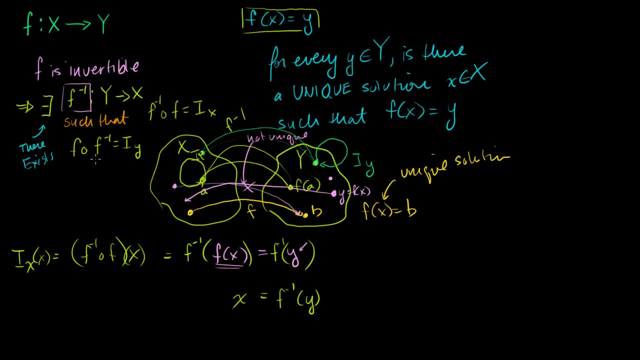 We used the definition of invertibility, that there exists this inverse function right there, And then we essentially applied the inverse function to both sides of this equation. Say: look, you give me any y, Any lowercase cursive y in this set y. 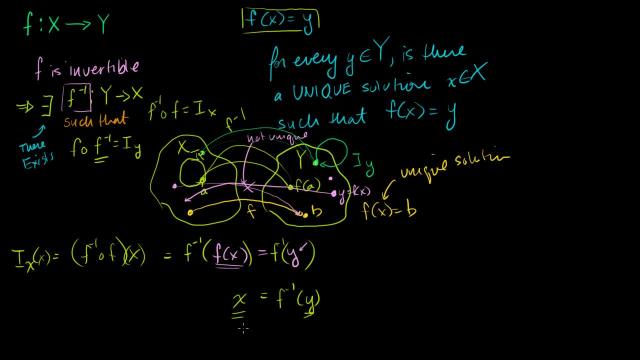 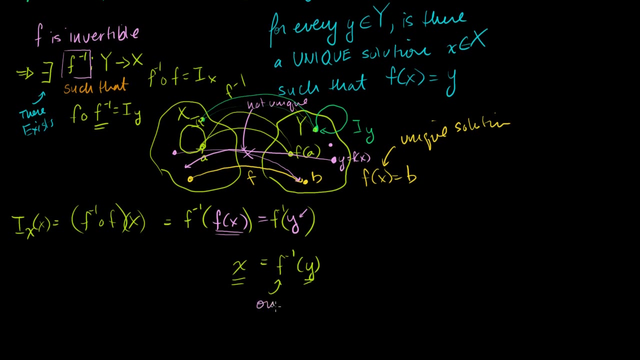 And I will find you a unique x. This is the only x that satisfies this equation. This is the only x. Remember if and how do I know? it's the only x Because this is the only possible inverse function, Only one inverse function for which this is true. 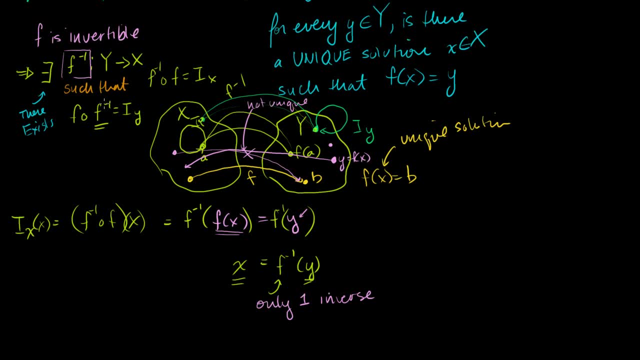 I proved that to you in the last video, That if f is invertible, it only has one unique inverse function. We tried before to have maybe two inverse functions, But we saw that they have to be the same thing. So since we only have one inverse function and it 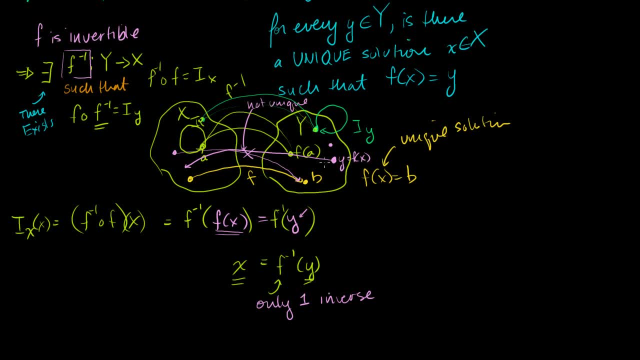 applies to anything in this big uppercase set y. we know we have a solution And because it's only one inverse function and functions only map to one value in this case, then we know this is a unique solution. So let's write this down. 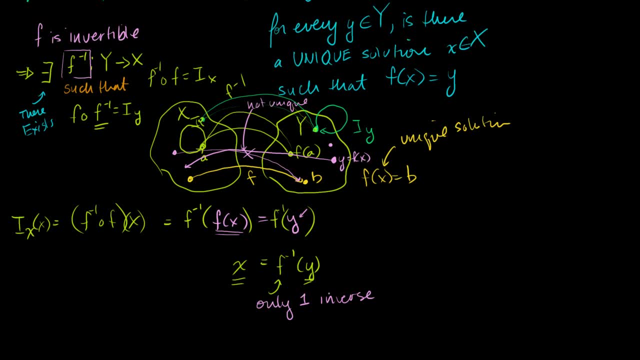 So we've established that if f is invertible- I'll do this in orange- If f is invertible, then the equation f of x is equal to y, for all that little v that looks like it's filled up with something. for all y, the member of our set y has a. 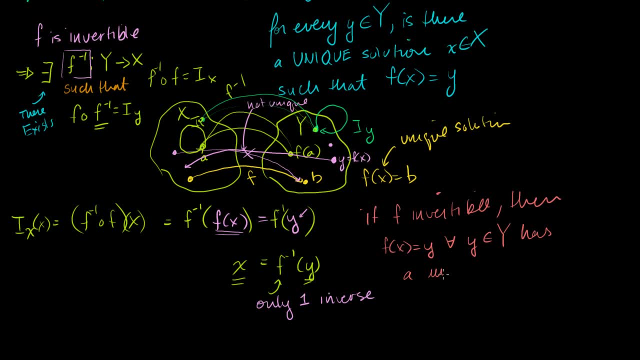 unique solution, And that unique solution, if you really care about it, is going to be the inverse function applied to y. It might seem like a bit of a no-brainer, but you can see, you have to be a little bit precise about it in order to. 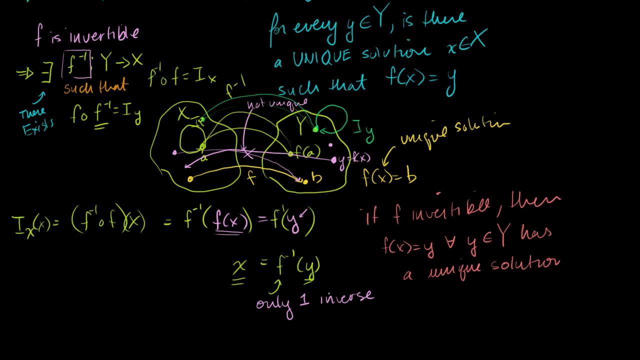 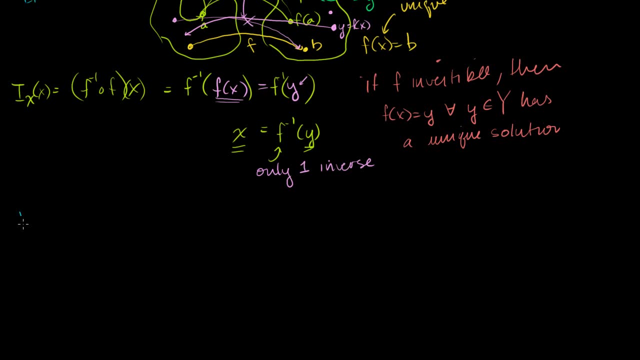 get to the point you want. Let's see if the opposite is true. Let's see if we start from the assumption that for all y that is a member of our set y, of our set y, that the solution, that the equation f 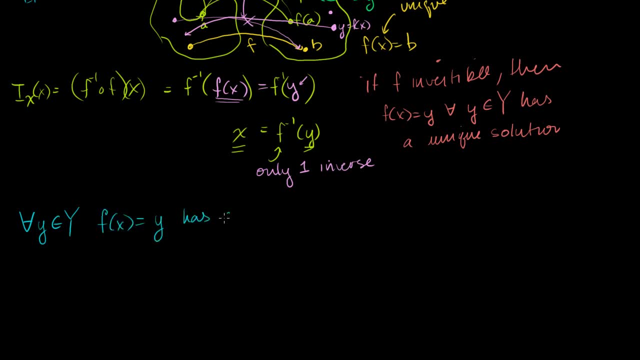 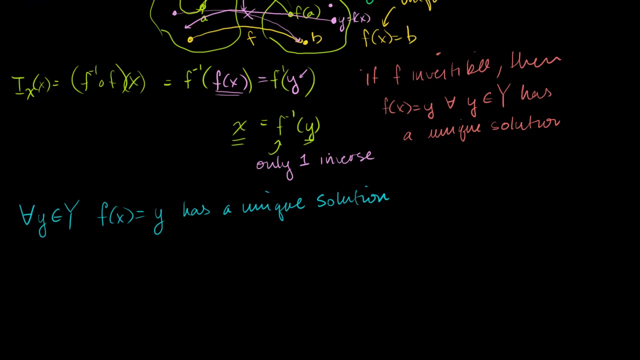 of x is equal to y has a unique solution. Let's assume this and see if it can get us the other way. Given this, we can prove invertibility, So let's think about it the first way. So we're saying that for any y, so let me draw my sets again. 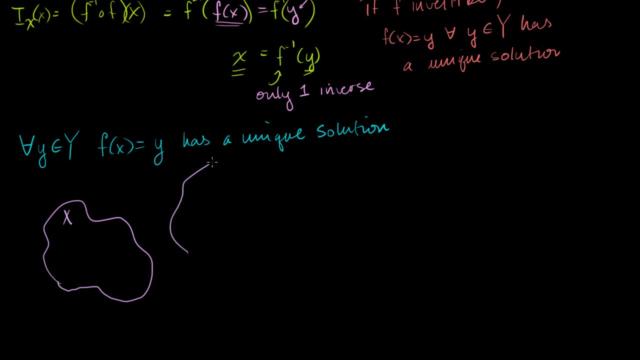 So this is my set x and this is my set y, right there. Now we're working for the assumption that you can pick any element in y right here, and then the equation right here has a unique solution. Let's call that unique solution. well, we could call: 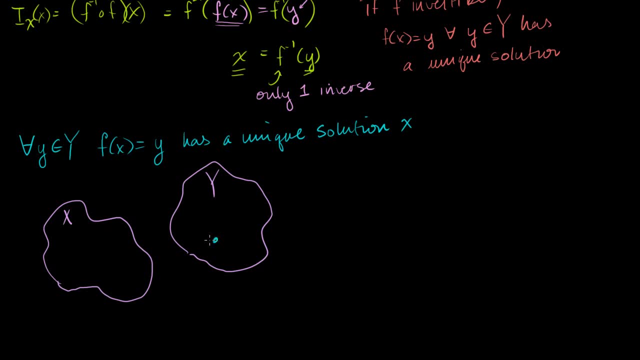 it whatever, but a unique solution: x. So you can pick any point here and I've given you- we're assuming now- that- look you pick a point in y, I can find you. I can find you some point in x, such that f of x is equal. 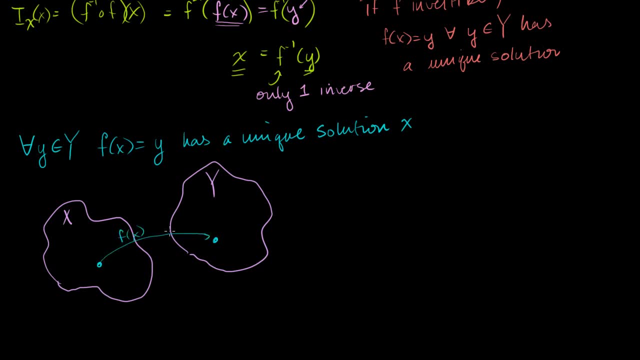 to y, and not only can I find that for you, that that is a unique solution. So, given that, let me define a new function. Let me define the function s. The function s is a mapping from y to x. It's a mapping from y to x. 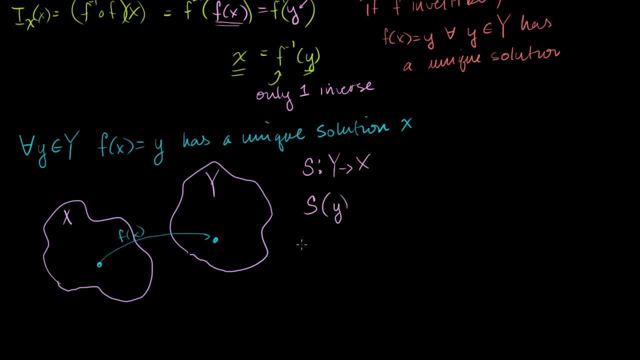 And s of, let's say s of y, where of course y is a member of our set, Set capital, y, s of y is equal to the unique solution in x to f of x is equal to y. Now you're saying: hey, Sal, that looks a little convoluted. 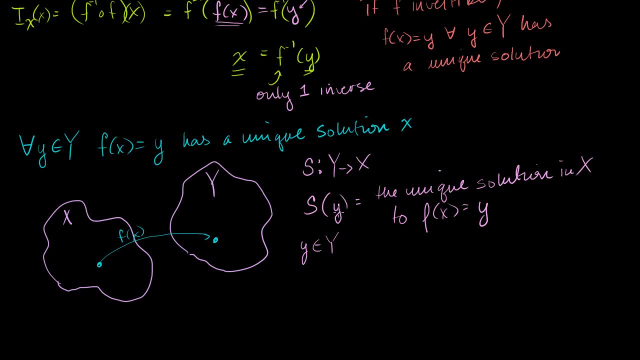 But think about it, this is a completely valid function definition. right, We're starting with the idea that you give me any y here, You give me any member of this set, and I can always find you a unique solution to this equation. 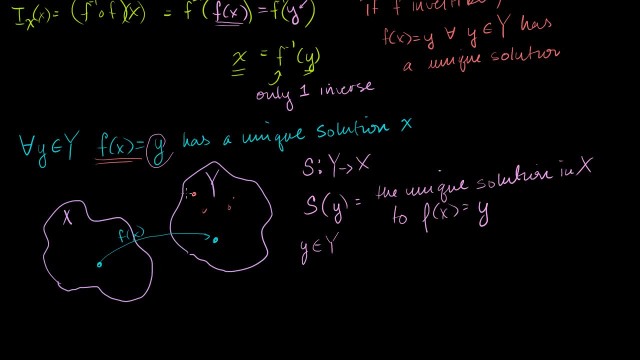 Well, OK, so that means that any guy here can be associated with a unique solution in the set x, where the unique solution is a unique solution to this equation here. So why don't I just define a function that says: look, I'm. 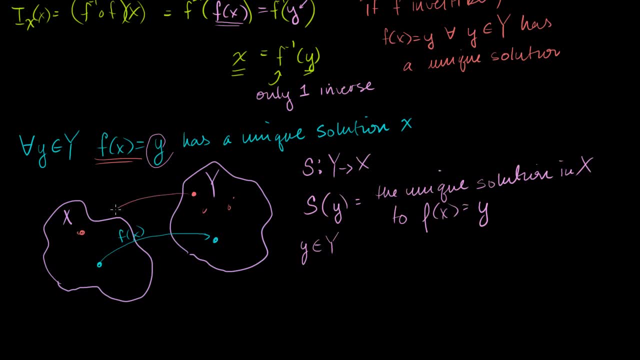 going to associate every member y with its unique solution to f of x is equal to y. That's how I'm defining this function right here. And, of course, this is a completely valid mapping from y to x. And we know that this only has one legitimate value, because 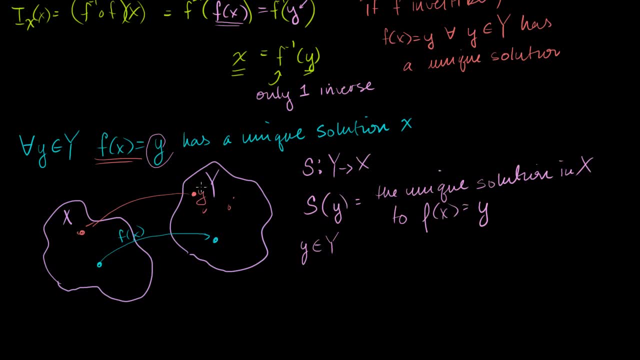 any value y. any lowercase value y in this set has a unique solution to f of x is equal to y, So this can only equal one value. So it's well-defined. Let's take some element here. Let me do a good color. 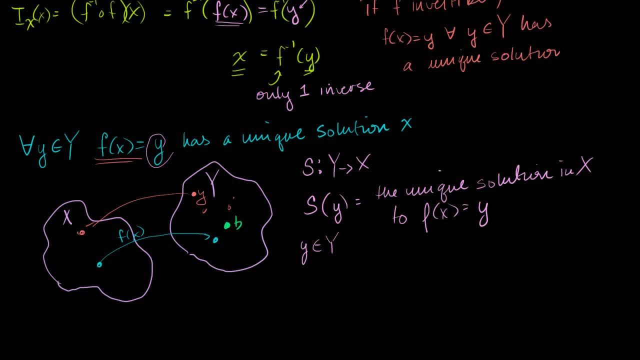 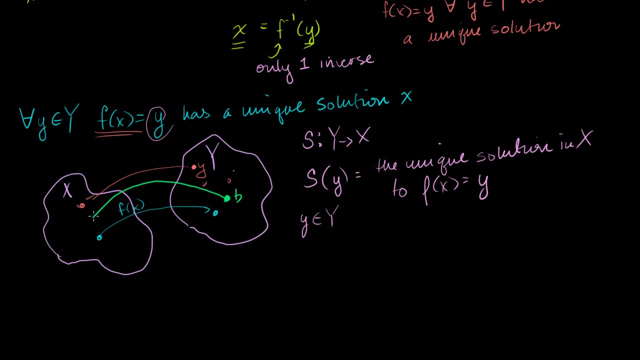 Let's say: this is b And b is a member of y, So let's just map it using our new function right here. So let's take it and map it. And this is s of b right here, which is a member of x. 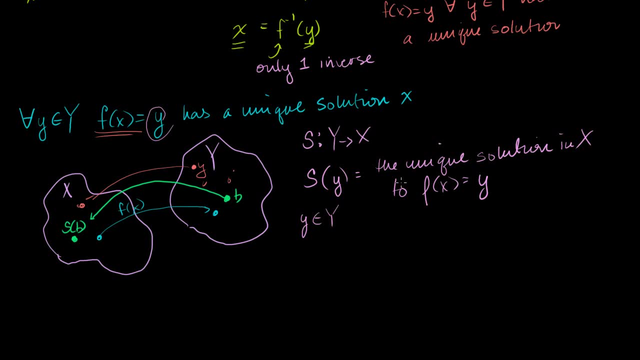 Now we know that s of b is a unique solution by definition. I know it seems a little circular, but it's not. We know that s of b is a solution, So we know that s of b is the unique solution. So this is a unique solution to f of x is equal to b. 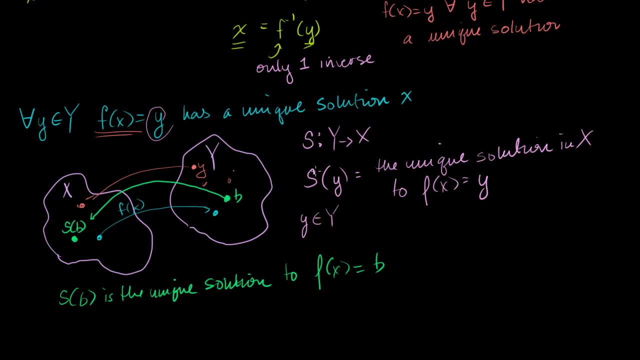 Well, if this is the case, we just got this because this is what this function does: It maps every y to the unique solution to this equation, Because we said that every y has a unique solution. So if this is the case, then what happens? if I take f of s, 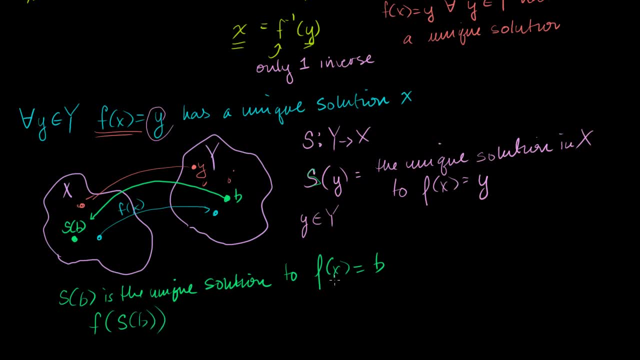 of b. Well, I just said, this is the unique solution to this. So if I put b- This guy in here, what am I going to get? I'm going to get b. Or another way of saying this is that the composition of f. 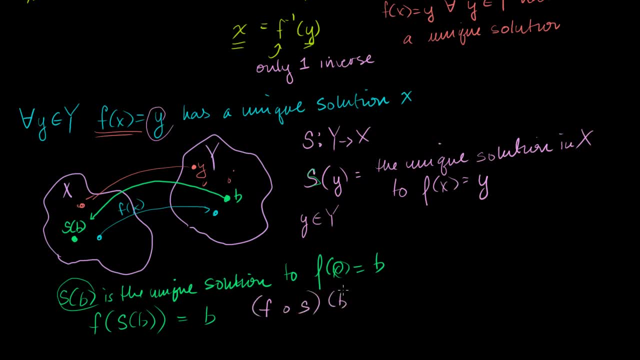 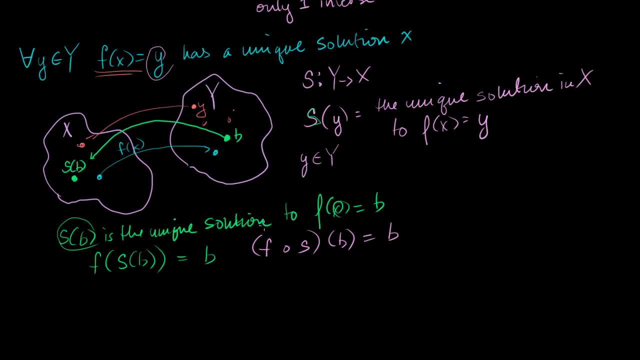 with s applied to b is equal to b. Or another way to say it is that when you take the composition of f with s, this is the same thing, Because if I apply s to b and then I apply f back to that, 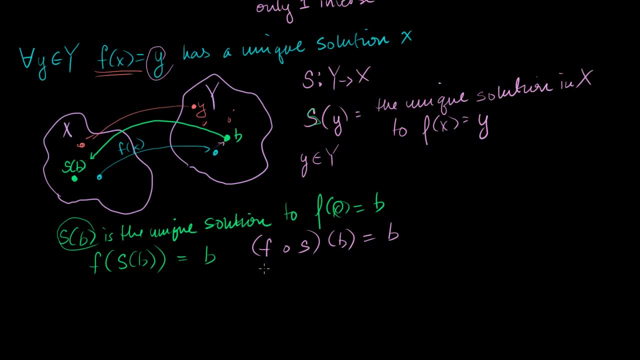 that's the composition. I just get back to b. That's what's happening here. So this is the same thing as the identity function. on y being applied to b, It's equal to b. So we can say that the composition. we can say that. 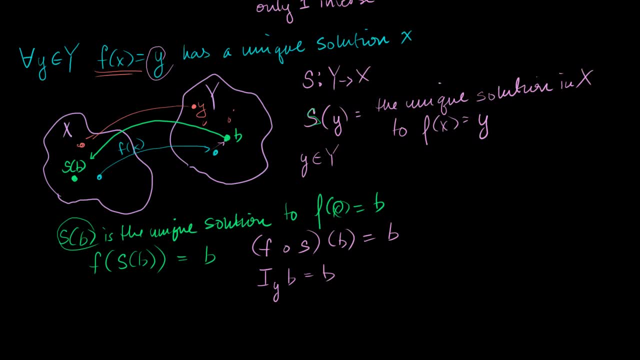 there exists And we know that this function exists or that we can always construct this, So we already know that this exists. This existed by me constructing it, but I've hopefully shown you that this is well-defined From our assumption that this always has a unique solution. 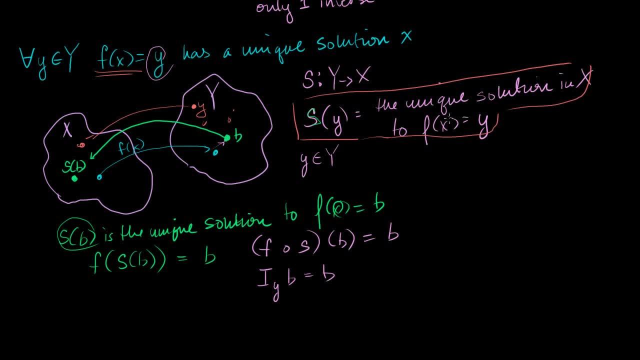 an x for any y. here I can define this in a fairly reasonable way. So it definitely exists. And not only does it exist, but we know that the composition of f with this function that I just constructed here is equal to the identity function on y. 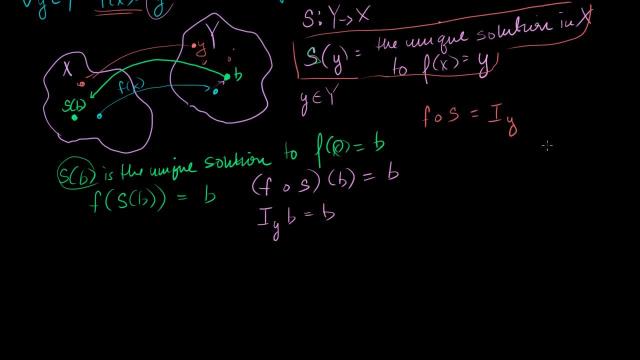 Now let's do another little experiment. Let's take a particular. Let me just draw our sets again. Let me take some. This is our set x, And let me take some. member of set x. call it a. Let me take my set y, right there. 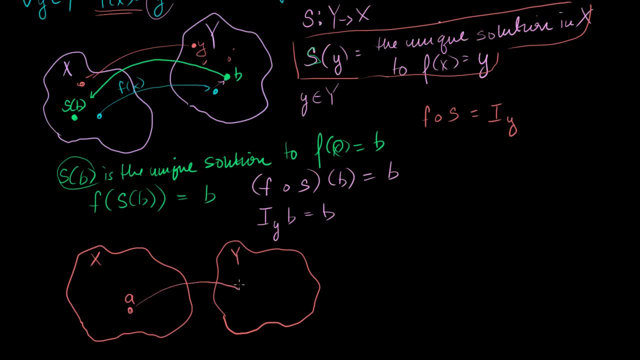 And so we can apply the function to a and we'll get a member of set y. Let's call that right there. Let's call that f of a, right there. Now, if I apply my magic function here, that always I can get you any member of set y and I'll give you the unique. 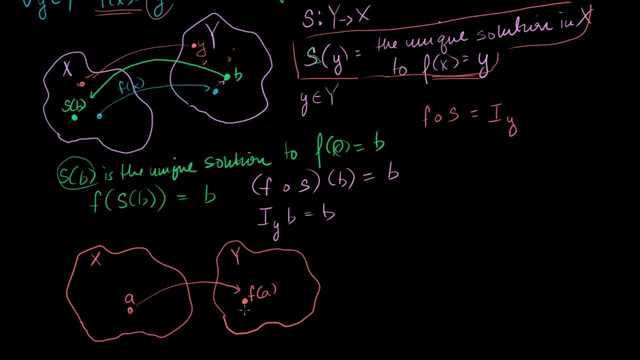 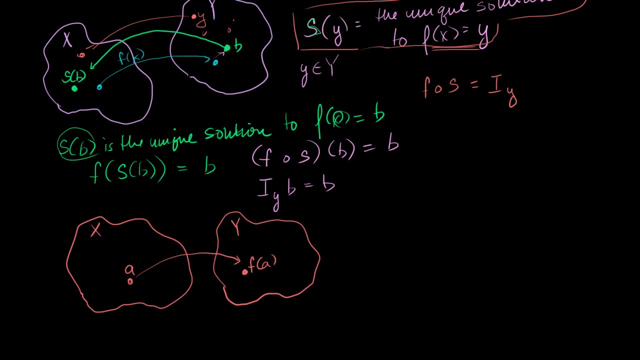 solution in x to this equation. So let me apply that to this. Let me apply s to this. So if I apply s to this, it'll give me the unique solution. Let me write this down. So if I apply s to this, I'm going to apply s to this. 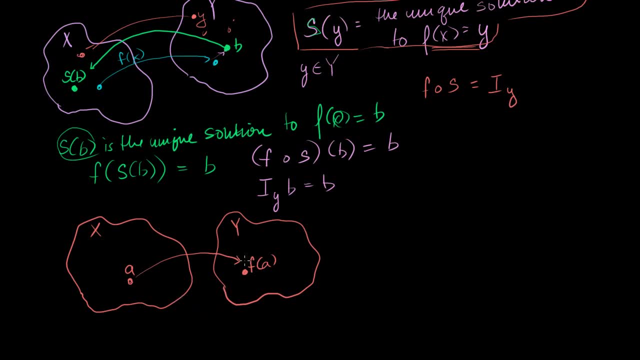 And maybe I shouldn't point it back at that. I don't want to imply that it necessarily points back at that, so let me apply s to that. So what is this going to point to? What is that point going to be right there? 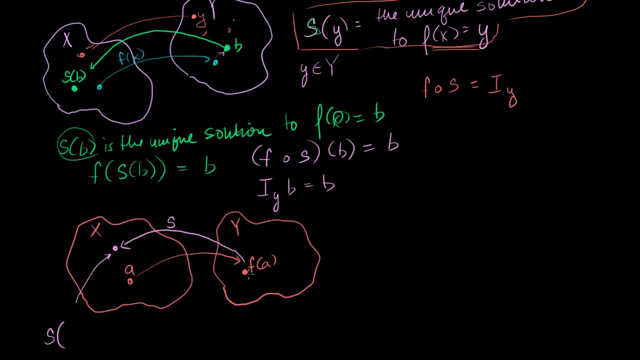 So that's going to be s of this point, which is f of a, which we know is the unique solution. So this is equal to the unique solution to the equation, to the equation f of a. f of x is equal to this y, right here. 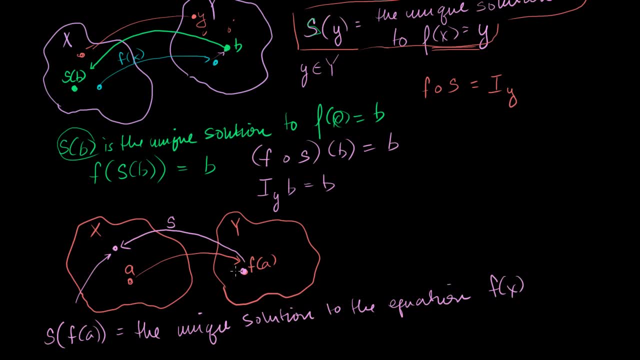 Or this y right here is just called f of a right. Remember: the mapping s just maps you from any member of a to the unique. solution to the equation f of x is equal to that. So this is the mapping from f of a to the unique. 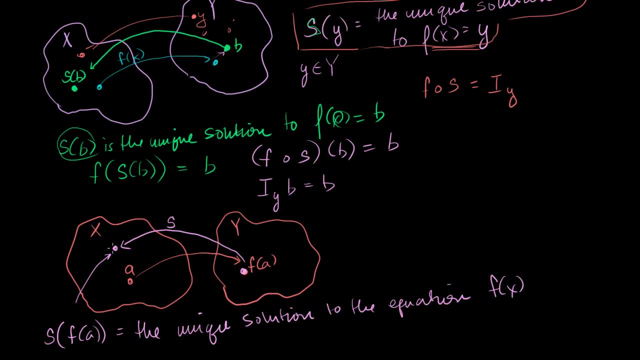 So this s of f of a is going to be a mapping to the or this right here is going to be the unique solution to the equation. f of x is equal to this member of y, And what's this member of y called? It's called f of a. 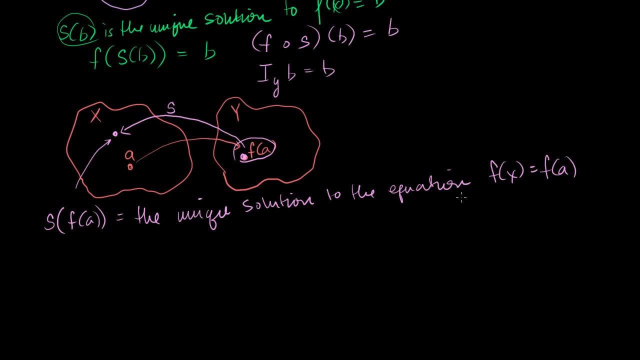 Well, what is? you could say this in a very convoluted way, but if I were to, just before you learned any linear algebra. if I said: look, if I have the equation f of x is equal to f of a, what is the unique solution to this? 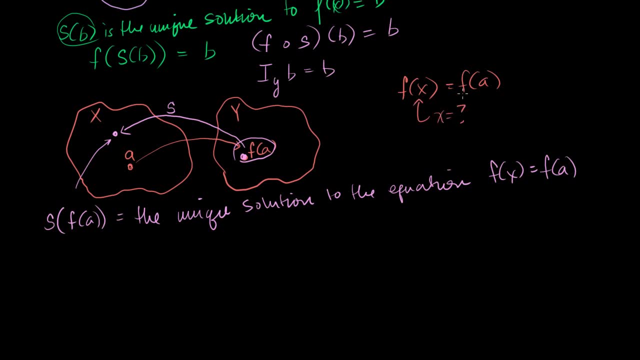 equation: What does x equal? Well, x would have to be equal to a, x would have to be equal to a. So the unique solution to the equation: f of x is equal to a, f of x is equal to f of a is equal to a. 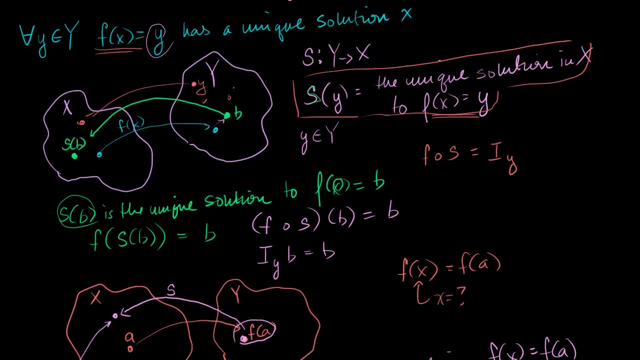 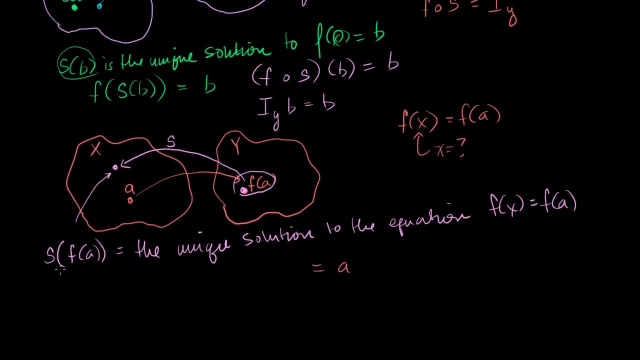 And we know that there's only one solution to that, because that was one of our starting assumptions. So this thing is equal to a, Or we could write s of f of a is equal to a, or that the composition of s with f is equal, or applied to a is. 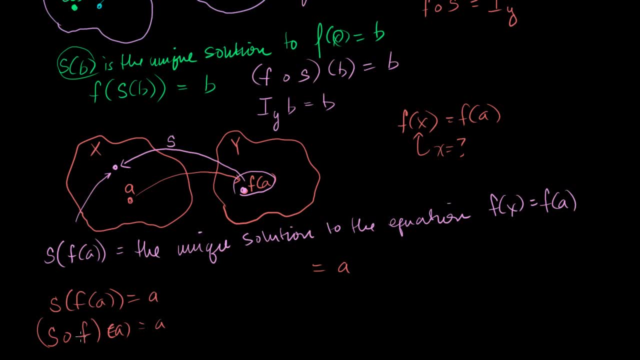 equal to a or that the composition of s with f is just the identity function on the set x. This is a mapping right here from x to x, So we could write that s: the composition of s with f is the identity on x. 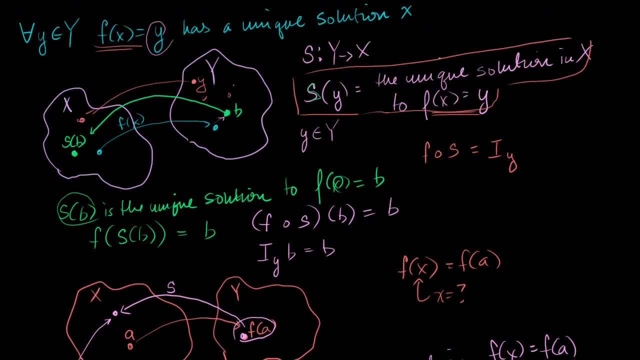 So what have we done so far? We started with the idea that you pick any y in our set capital, Y here, and we're going to have a unique solution: x, such that this is true, Such that f of x is equal to y. 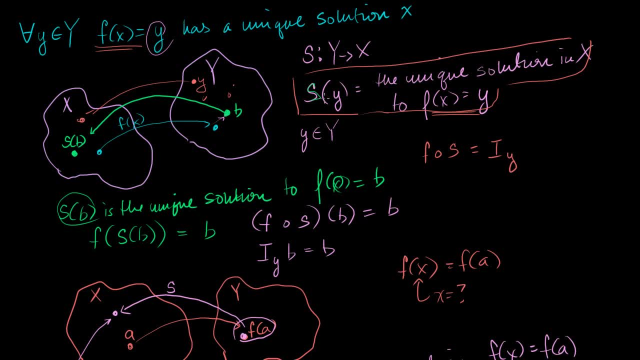 That's what the assumption we started off with. We constructed this function s that immediately maps any member here with its unique solution to this equation. Fair enough. Now, from that we say, OK, this definitely exists. Not only does it exist, but we figured out that the 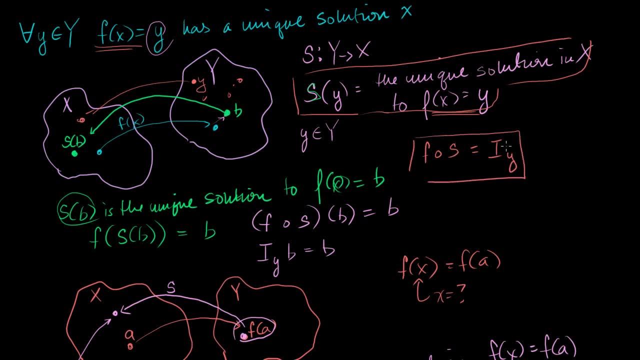 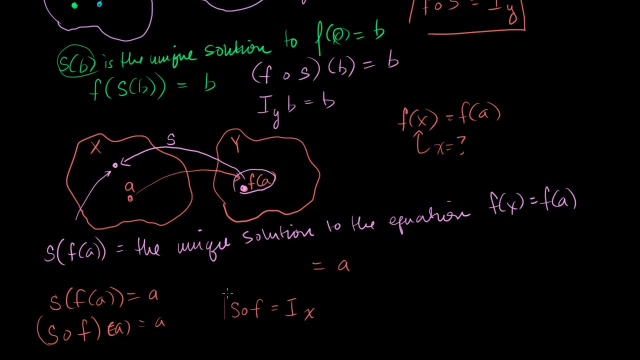 composition of f with our constructed function is equal to the identity on the set y. And then we also learned that the composition of s with f is the identity function. Let me write this. So we learned this. and we also learned that the composition of f with s is equal to the identity on y. 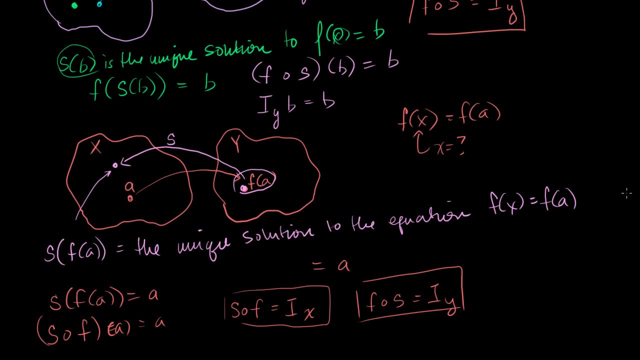 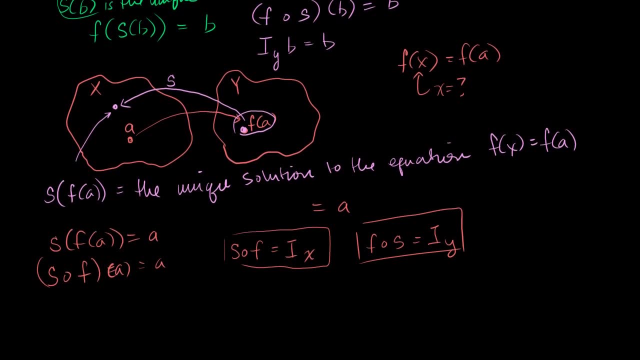 And s clearly exists because I constructed it and we know it's well-defined because for every y here there is a solution to this. So, given that I was able to find for my function f, I was able to find a function, that these two things are true. 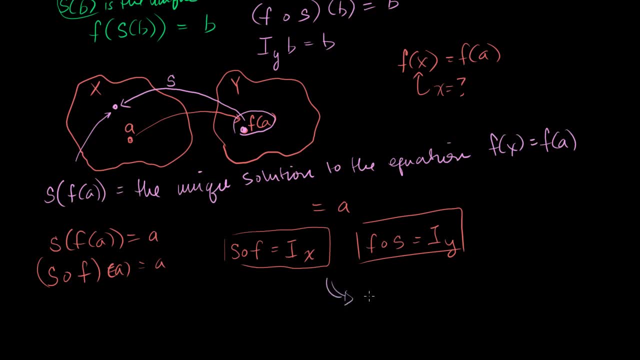 this is, by definition, What it means to be invertible, to be invertible, Remember. so this means that f is invertible. Remember f being invertible. in order for f to be invertible, that means that there must exist some function. 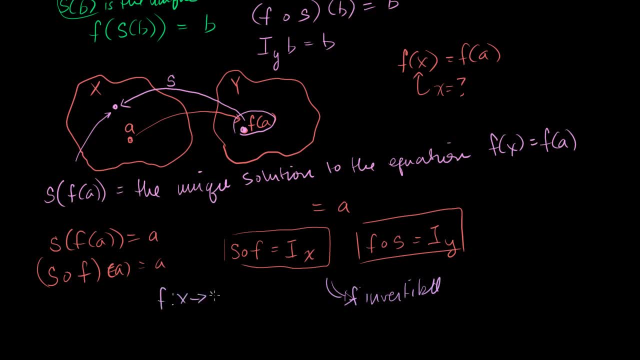 from. so if f is a mapping from x to y, invertibility means that there must be some function, f inverse, that is, a mapping from y to x, such that so I could write: there exists a function such that the inverse function composed with 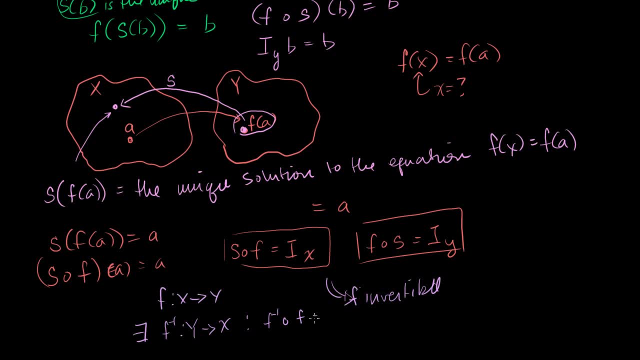 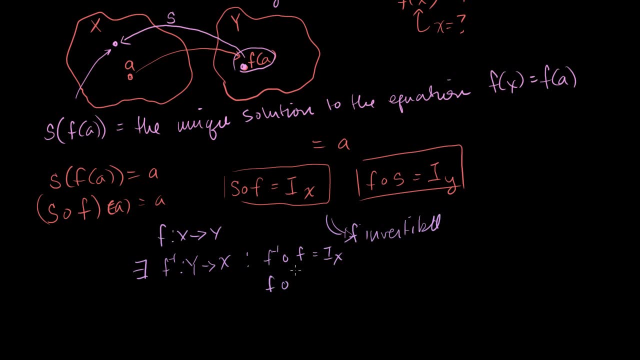 our function should be equal to the identity on x and the function in the composition of the function with the inverse function should be the identity on y. Well, we just found a function. It exists, And that function is s, where both of these things are true. 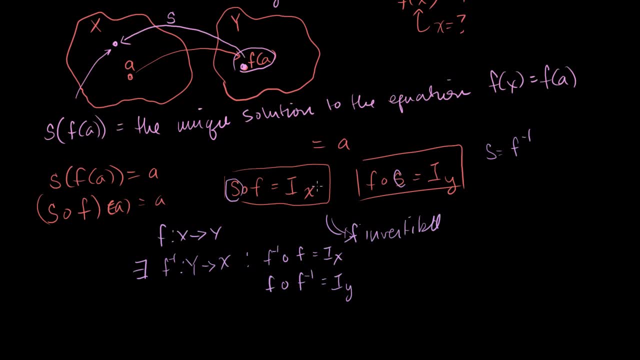 We can say that s is a mapping function. We can say that s is a mapping function. We can say that s is a mapping function. We can say that s is equal to f inverse, So f is definitely invertible. So hopefully you found this satisfying. 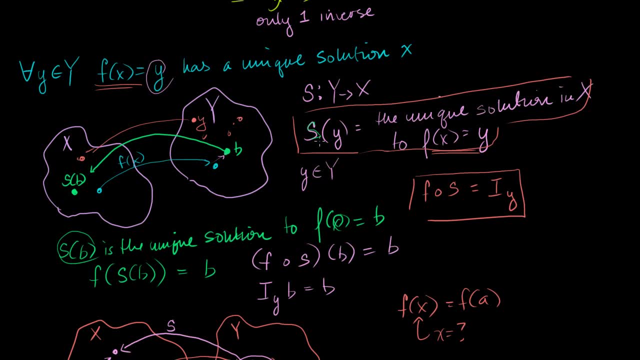 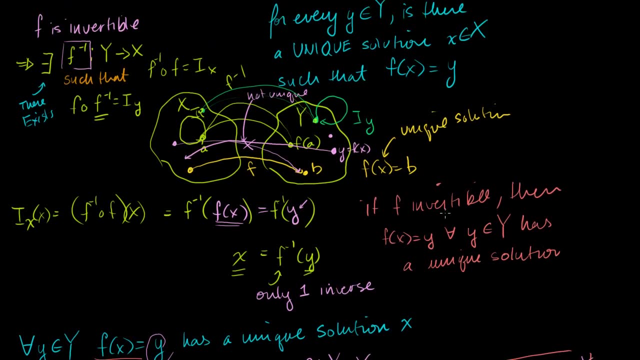 This proof is very subtle and very nuanced because we kind of keep bouncing between our sets x and y, But what we've shown is that if f is in the beginning part of this video, we showed that if f is invertible, then for 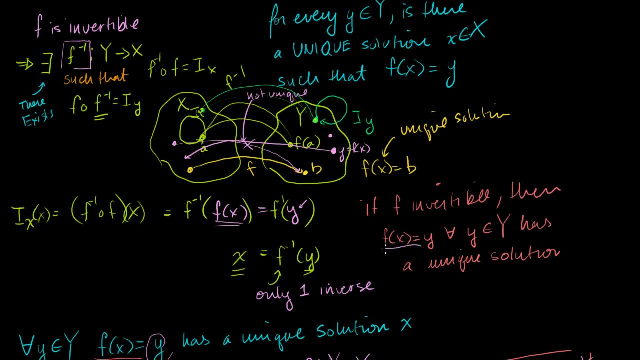 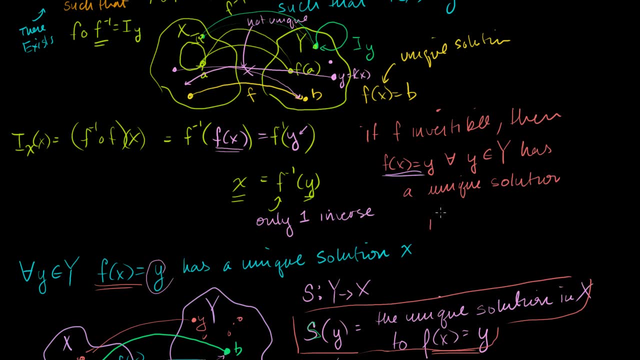 any y. there is a unique solution to the equation f of x equals y, And in the second part of the video we showed it that the other way occurred. The other way is true That if- let me put it this way- that if for all y a, 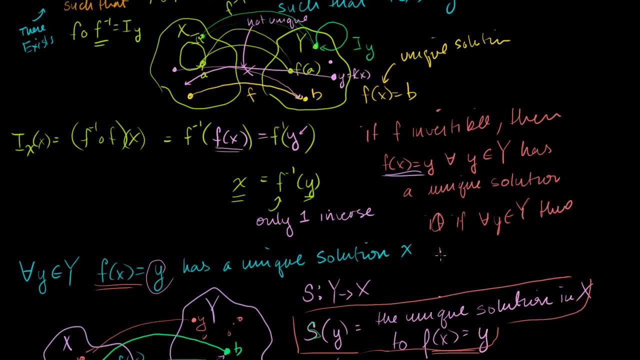 member of capital Y. there is a unique solution to f: of x is equal to x, then f is invertible. So the fact that both of these assumptions are invertible is that if f is invertible, then f is invertible. 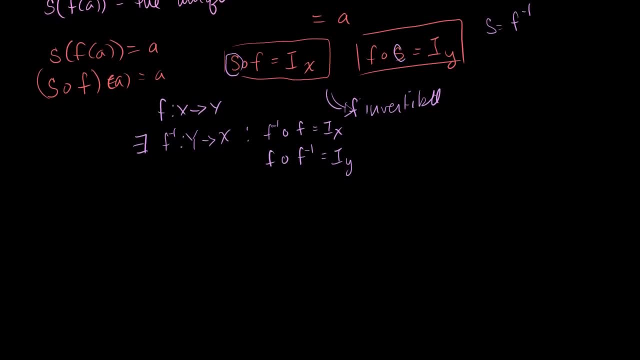 And if both of these assumptions imply each other, we can write our final conclusion of the video That f being invertible. if f, which is a mapping from x to y, is invertible, this is true if, and only if, And we could write that either as a two-way arrow or we could.